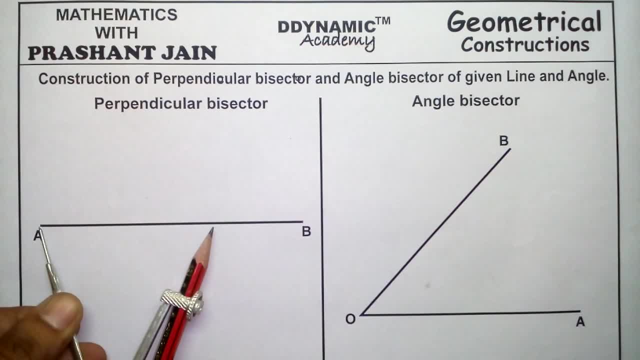 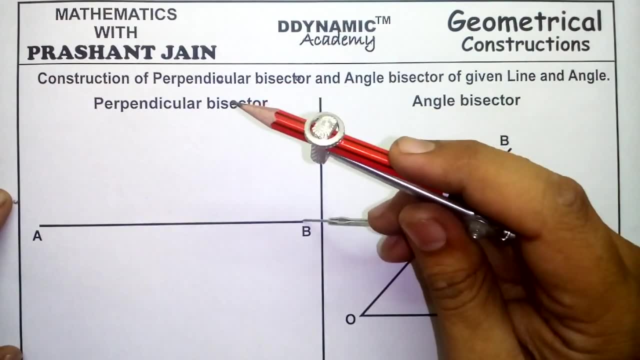 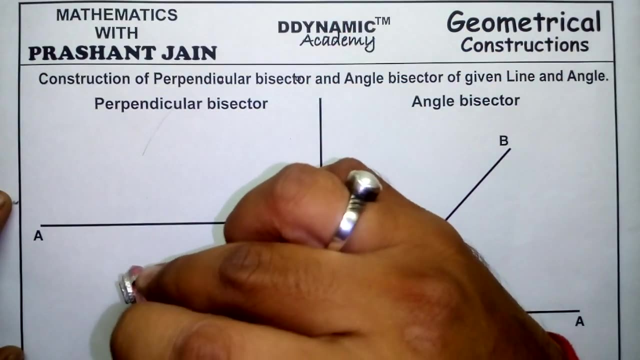 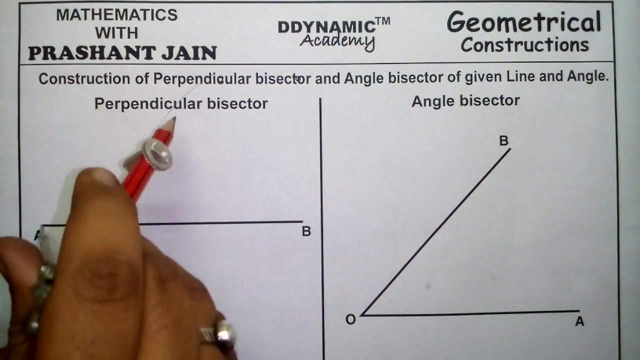 compass like this: now, after open the compass, just put the needle of the compass on the point B and make an arc on the above part of the line segment, as well as on the below part of the line segment, similar part. you will do with the point A. make an arc on the above part as well as on the. 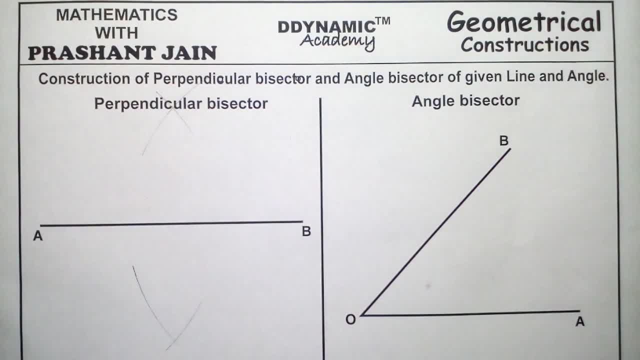 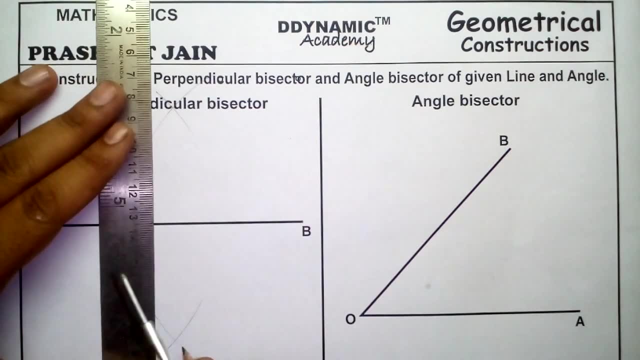 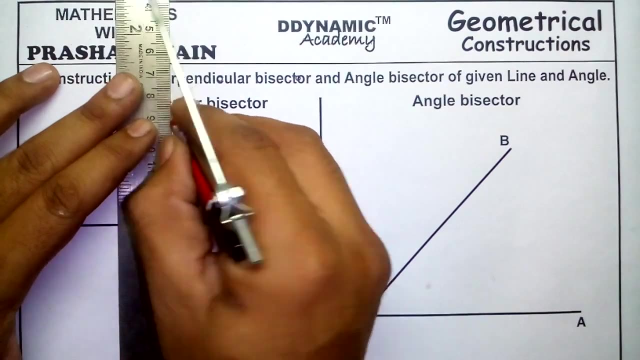 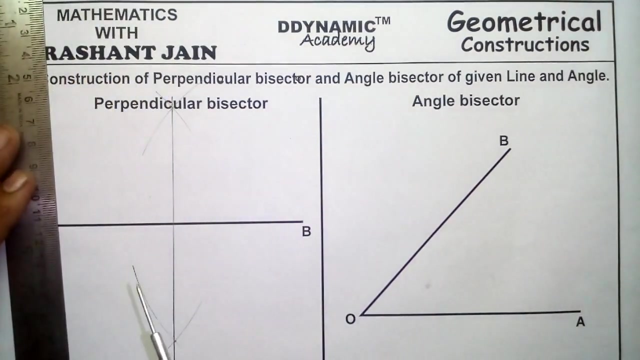 B below part of the line segment where these two arc intersect each other. just join with the help of the scale. please be aware that these intersecting points must meet with line segment. draw the line segment where this line intersect, the point m. this is the perpendicular bisector. it means: 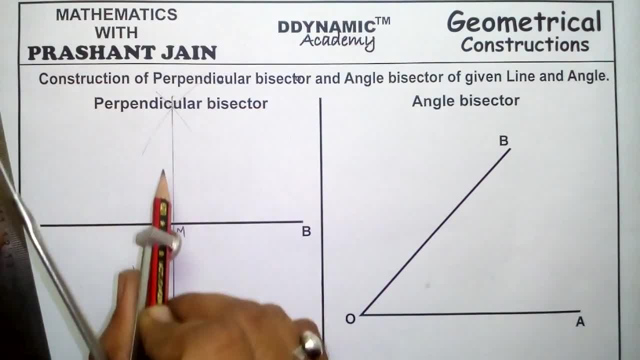 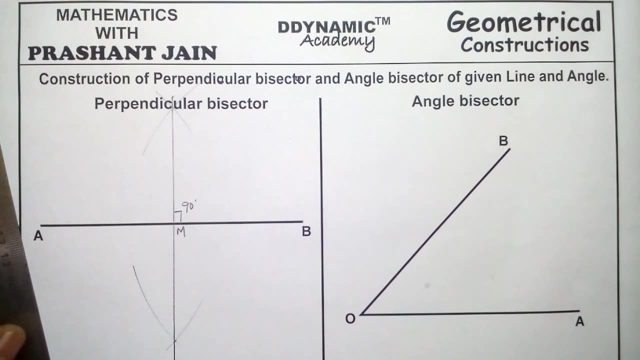 am is equals to mb, as well as this angle is equals to 90 degree. this is the way how to draw the perpendicular bisector. now we draw the angle bisector. angle bisector means bisect a given angle if we don't know how much of given measurement is. 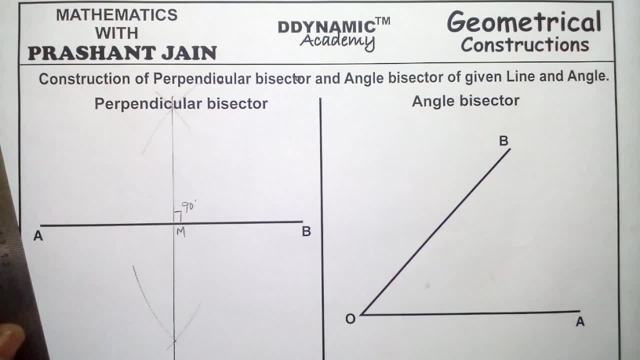 just, we know that there are angle a or b. we just take a compass, open the compass and put the needle on the point o. just make an arc of any of any line segment. sorry, yes, now put the compass on the other part, which will be on the line segment oa, just. 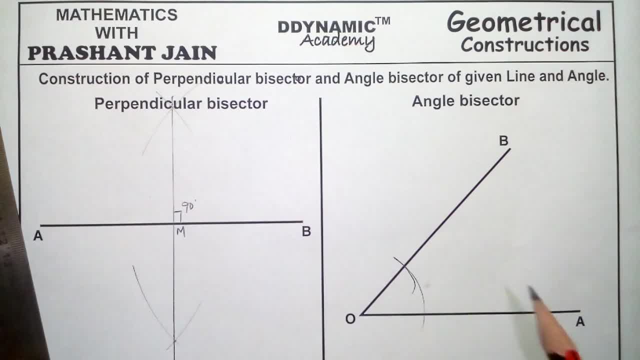 if you want, then you can open the compass little bit greater. just put this the middle, on the this part, and make an arc. put the needle on the other point, on the line segment a, b, and make an arc where these line in these arcs intersect with each other. just join with the point.